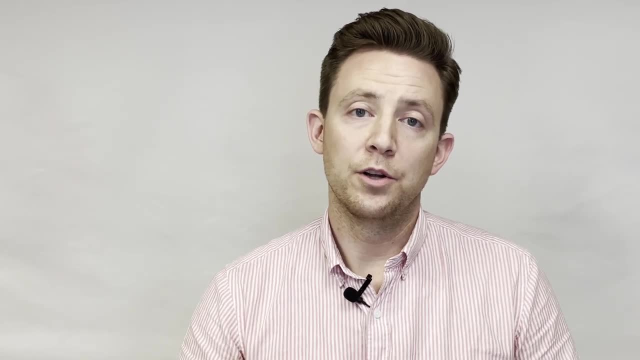 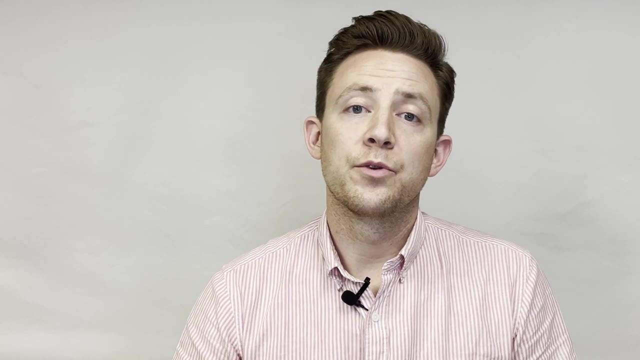 of Python. As you're going to see with lots of these courses, one critical piece is having the materials and sample code that you can start to use and run with right from the beginning. This course is no different. There's great notebooks or Jupyter notebooks that you can. 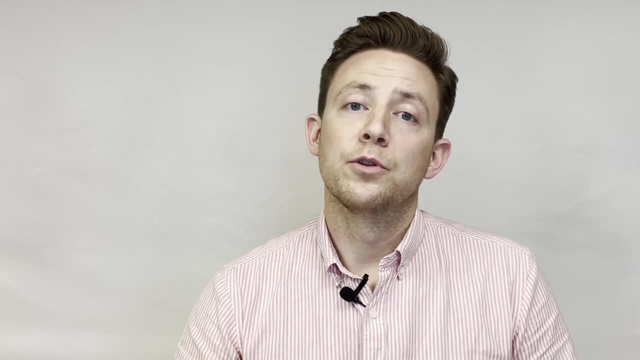 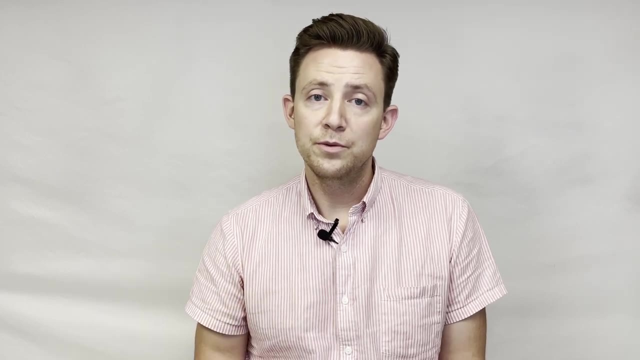 use to actually pull from and start using right in your library, In your local environment. So the four areas I'm going to look at in each of these courses are their accessibility, How easy are they to use, their geospatial focus or how much of the 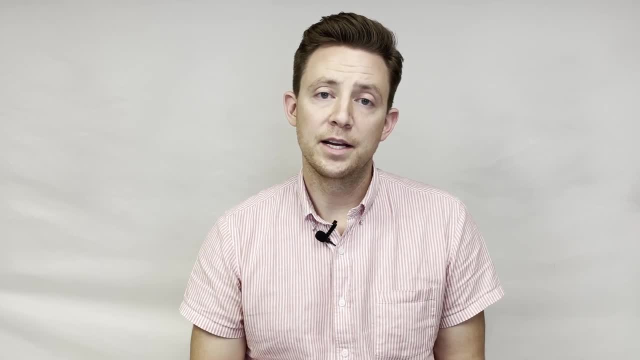 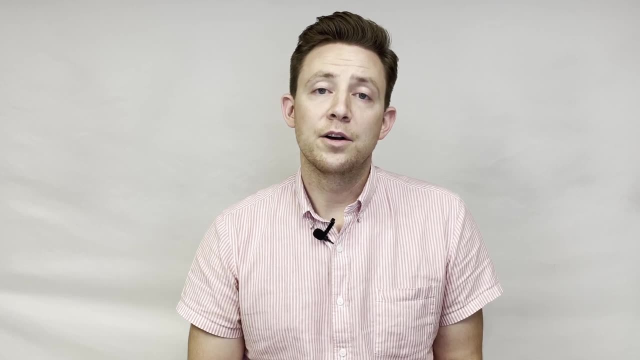 content is focused specifically on geospatial or modern GIS. I'm also going to look at the clarity of the content: How easy is it to learn and how clear are the concepts being explained, and also the completeness. This is definitely a beginner tutorial, So 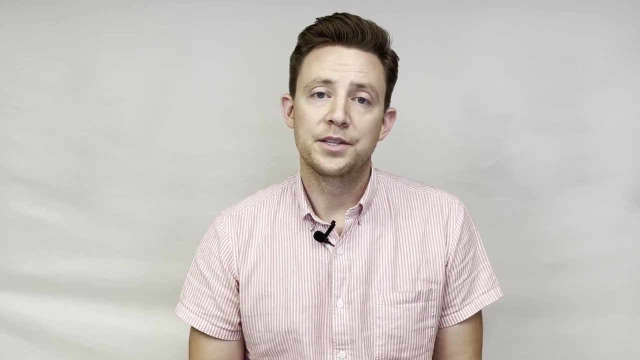 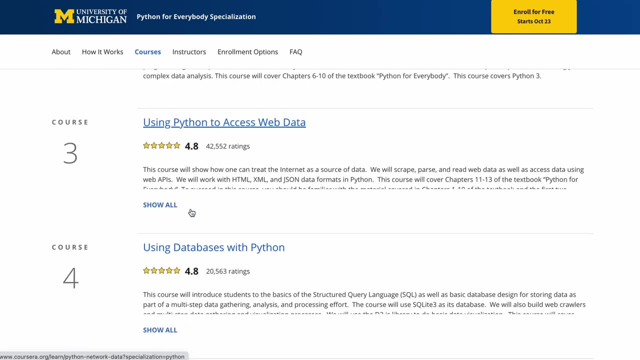 if you have not started or used Python before, this is a great place to start. Another course I think is pretty interesting is called Python for Everybody. It's brought to us by Coursera and the University of Michigan, So this is also a beginner course focused on generic Python skills. It's well. 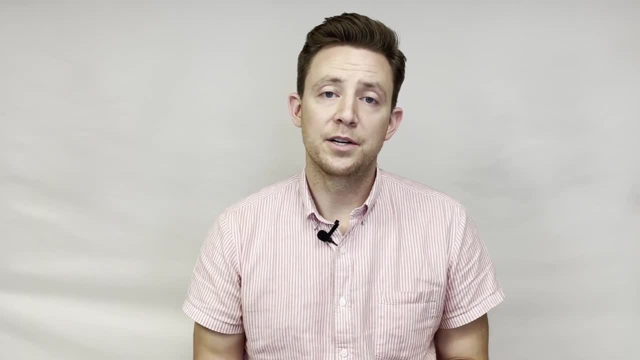 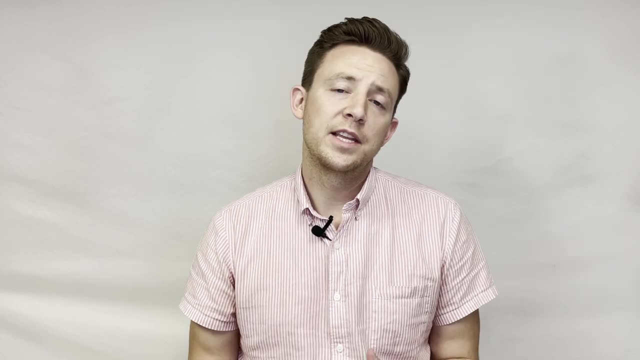 trusted in the data community and I think is a great place to start. So, with that said, I think it's really focused on basic data, fundamentals, things like web scraping and other tools. So if you're interested in that, check it out. But you can pick up some of these concepts with the other. 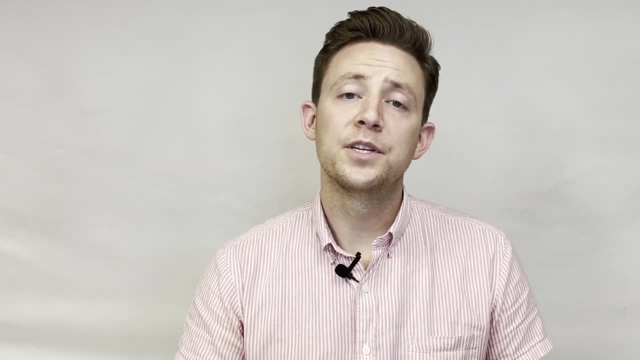 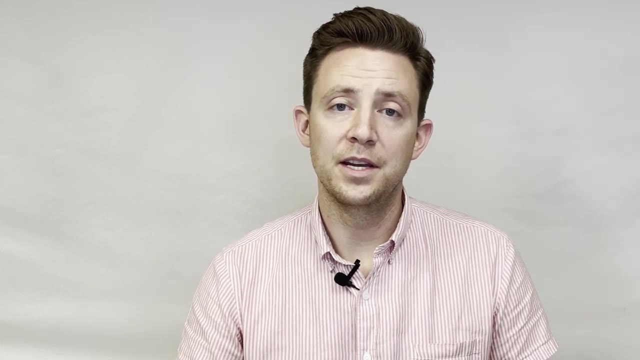 courses too. Now that we have some of the basic Python courses laid out, I'm going to focus on the most specific courses next. This next course comes from us, from our friends at the University of Helsinki, And, if you're watching this, a big thank you for all you have contributed to the. 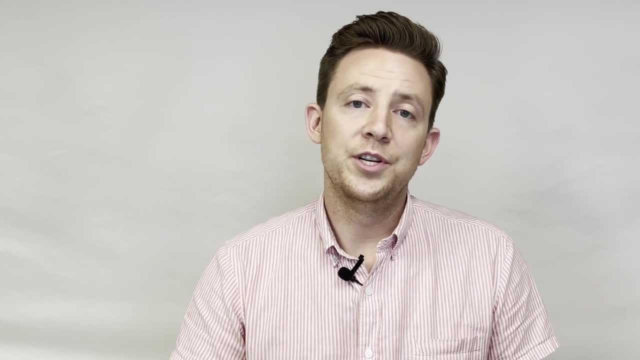 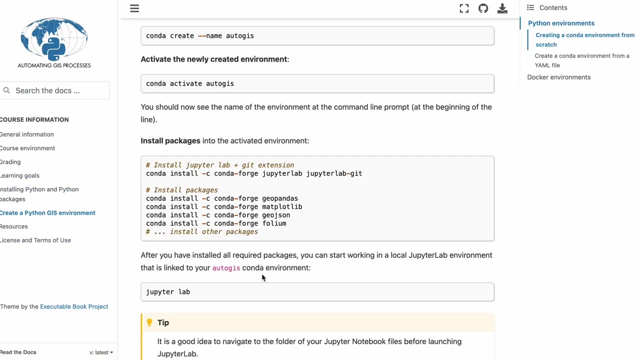 geospatial community over the years. This course is called Automating GIS Processes and I recommend it to anyone who's starting or getting a start in geospatial and wants to use Python. What I like most about this course: it's highly readable. It's going to give you a very good introduction. 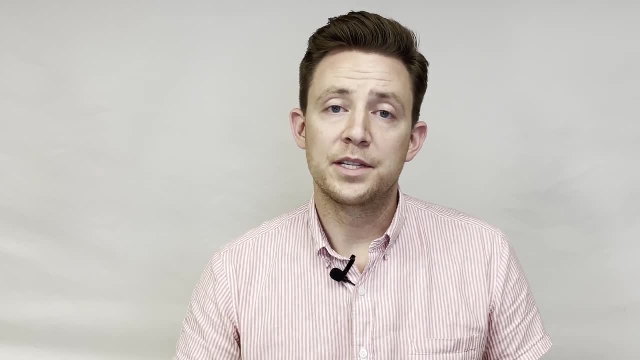 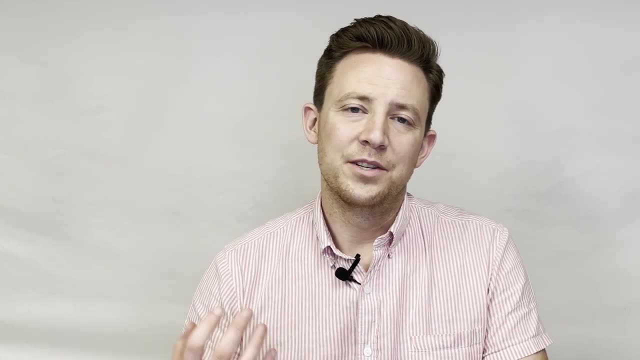 to Python and you should be walking away being able to complete some of the things you do in GeoGIS or different desktop software right in Python. This also focuses on other topics such as Python for QGIS and using raster data, But overall it's super readable and a great course that I think. 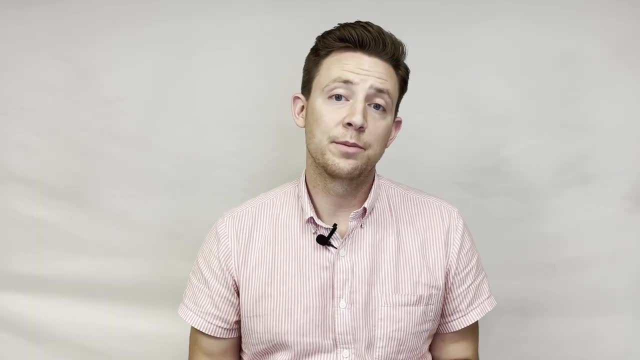 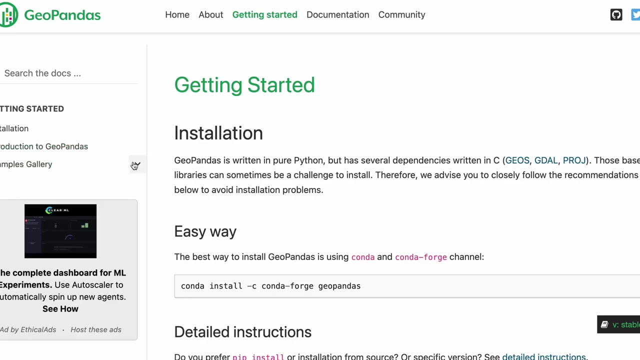 is an excellent starting point for geospatial Python. So the second course I'm going to recommend, well, isn't actually a course at all. It's actually jumping into the GeoPandas documentation. If you are going to get into programming, you will need to learn how to use. 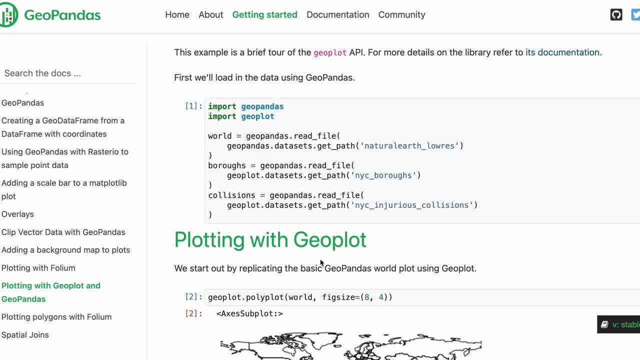 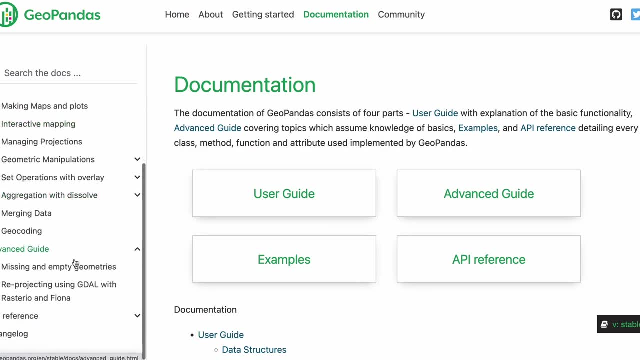 documentation And for me it's one of the fundamental skills that really helped me advance my programming skills forward. If you can really learn how to read docs and understand what they're saying, this really helps you understand what's happening under the hood. being able to quickly 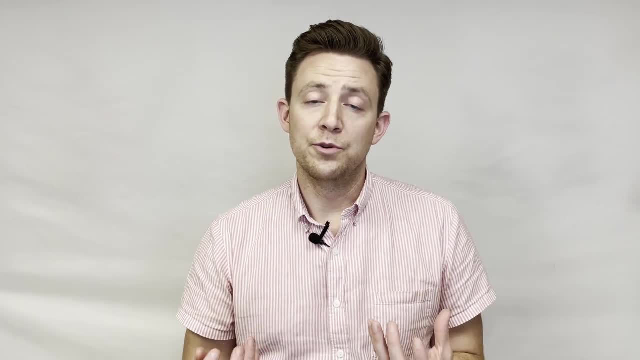 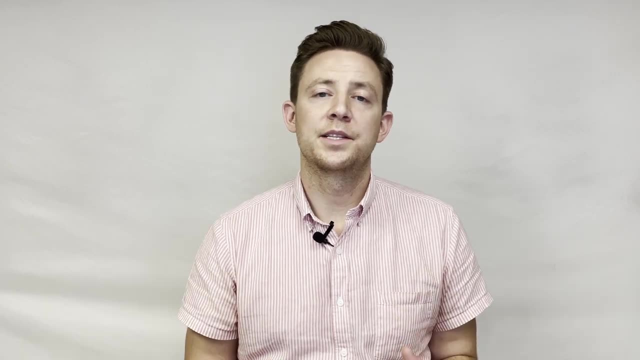 debug if there are problems with your code and ultimately use the tutorials and tools written by the people that are actually building that library themselves. GeoPandas documentation has excellent tutorials that help you jump right in and start using the language. It's one of the foundational 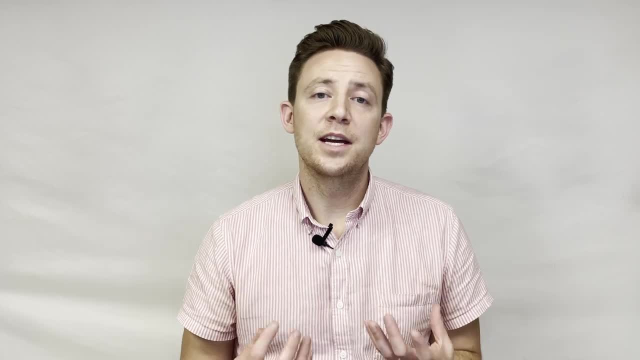 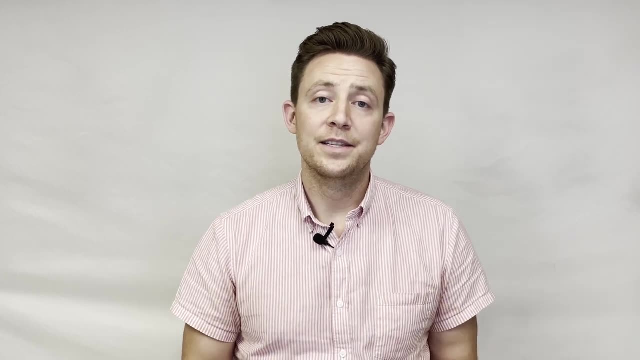 libraries for geospatial work. no matter what you're doing- And these are key concepts you will need to learn moving forward- GeoPandas helps you do everything, from reading and writing data, performing different analyses, connecting to other database tools, and doing that all in a geospatial setting. The tutorials: 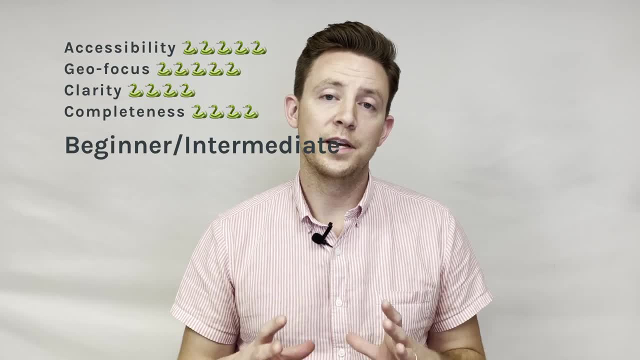 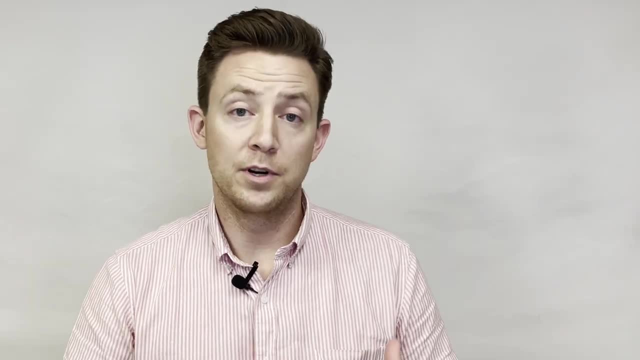 range from beginner to intermediate, but they're all focused and they're all going to be pieces that you can use in your geospatial Python path going forward. This third tool is actually one of my favorite advancements in geospatial Python- or, frankly, modern GIS- that I've seen in the last 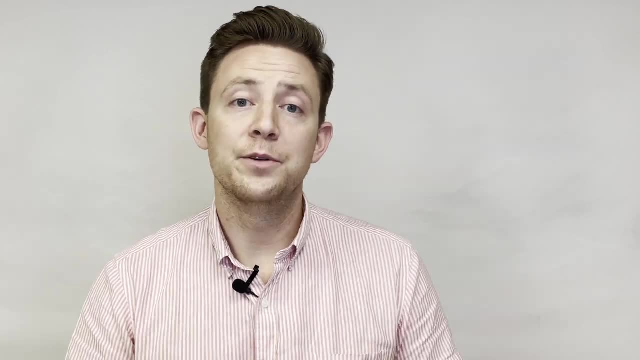 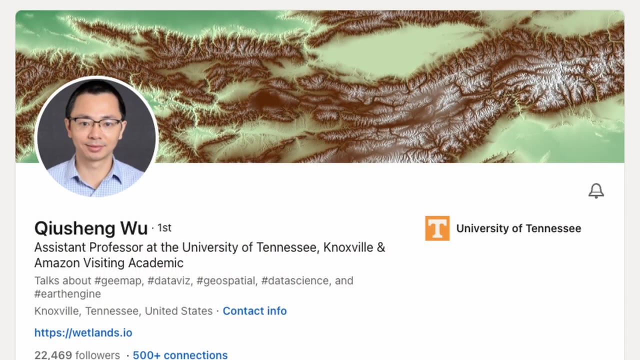 couple of years. It's called Leafmap and I think it's going to be one of the additional pieces for geospatial moving forward. This truly amazing library is maintained by Professor Kui-Hsien Wu from the University of Tennessee. I liken Leafmap to a complete 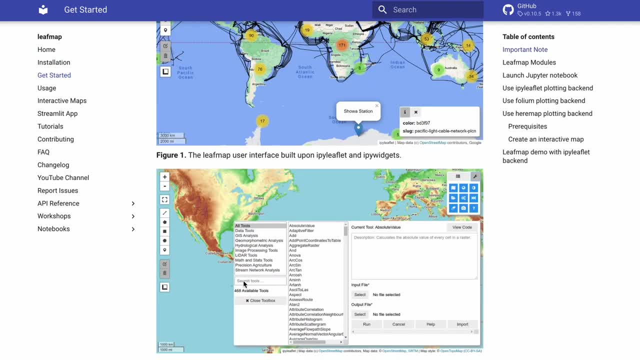 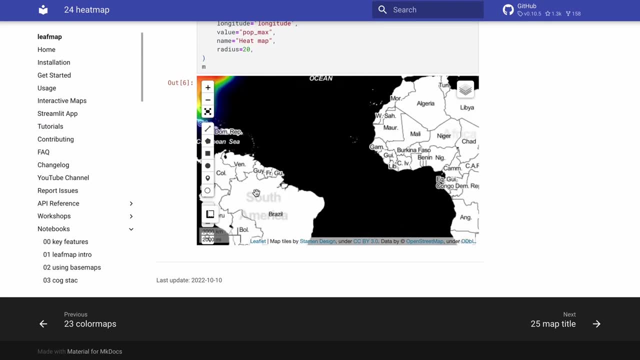 and when I say complete, a really complete geospatial toolkit in Python. This means that you can do everything from raster data to using vector data. You can read data from many different sources, perform visualization, do really advanced raster analysis or vector analysis. 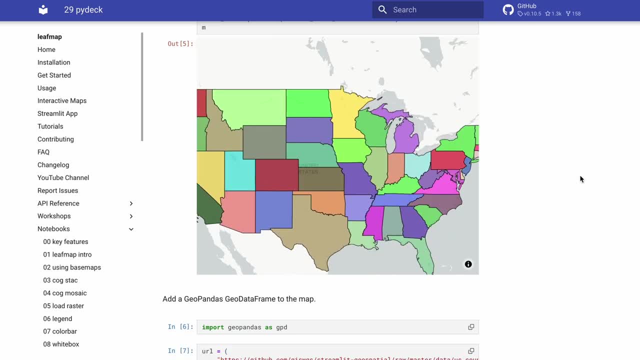 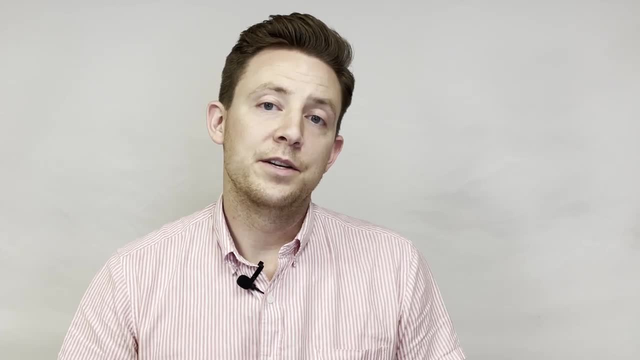 and you can do anything you want to do. If you're looking for a good resource for GeoPandas, I mean, the possibilities are really limitless with this library. Professor Wu also does an amazing job building great resources to help you use this, If you haven't checked him out. 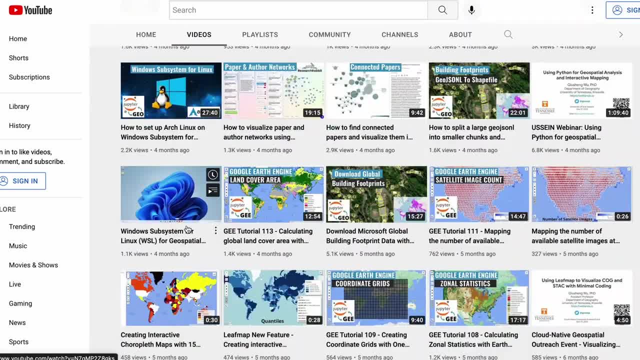 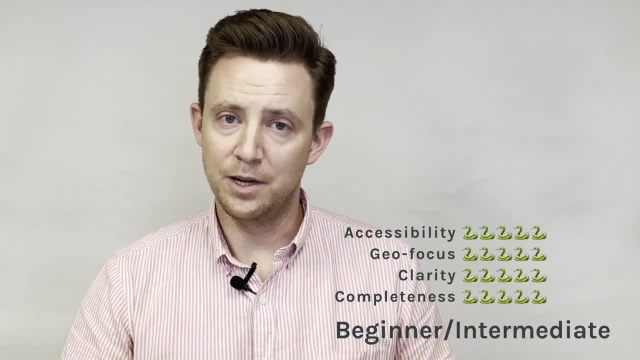 his YouTube page is here and I think he has so many amazing tutorials to help you get started. The documentation is really excellent as well. There's great tutorials that help you do just about anything you might want to do. Once again, these range from beginner to intermediate, but they 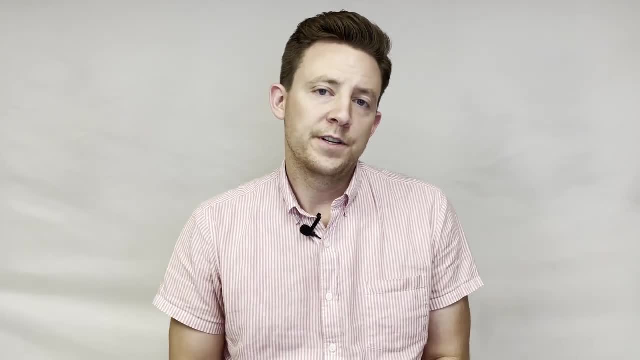 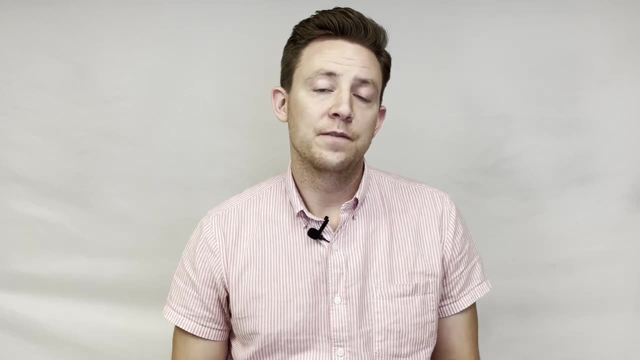 all focus on geospatial and they wrap in other libraries, like GeoPandas, that you're probably already using. Next is a course from Professor Danny Arribas-Bell from the University of Liverpool. It's a geographic data science course, and I think it's one of the best courses on spatial data science. 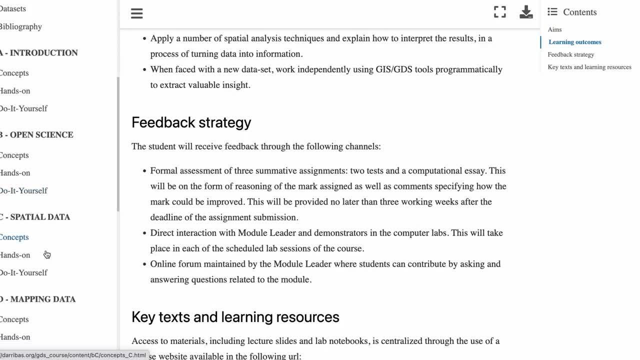 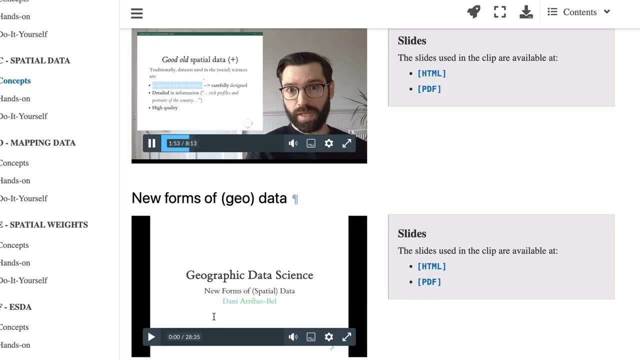 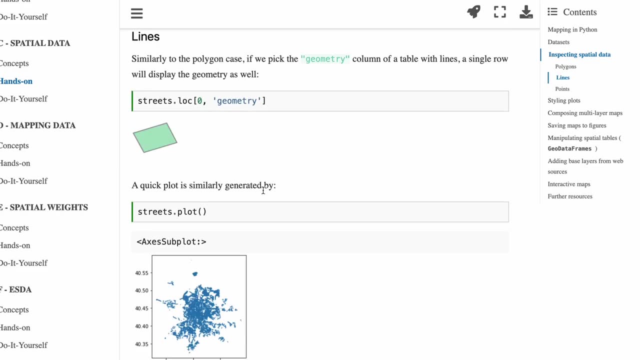 Dives into some key foundational elements. if you want to do more statistical analysis and use one of the best libraries out there, of which he's a contributor, called PyCell or the Python Spatial Analysis Library. This course has been taught many times and it's from one of the best sources and one of the best minds in spatial data science. 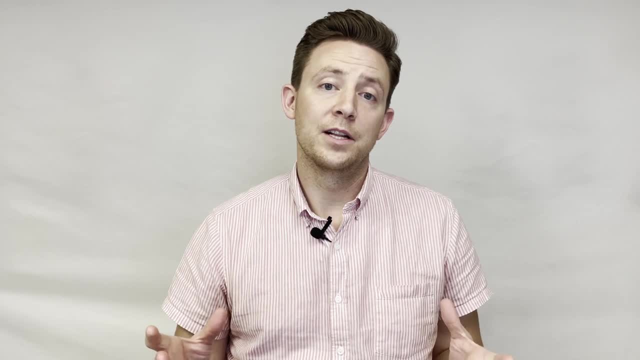 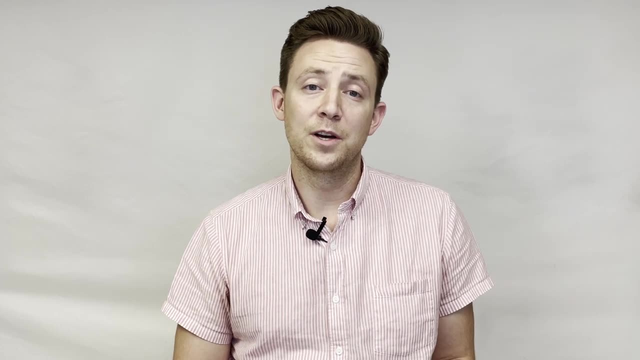 So this is a great place to go and thankfully, it's free and available to everyone to start using. This course is clear, it's concise, it has sample notebooks and it has an edition of videos as well for you to get started. I'd rank this more into the intermediate. almost some parts are into the. 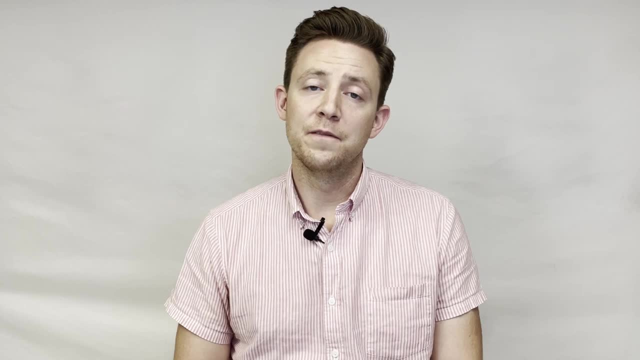 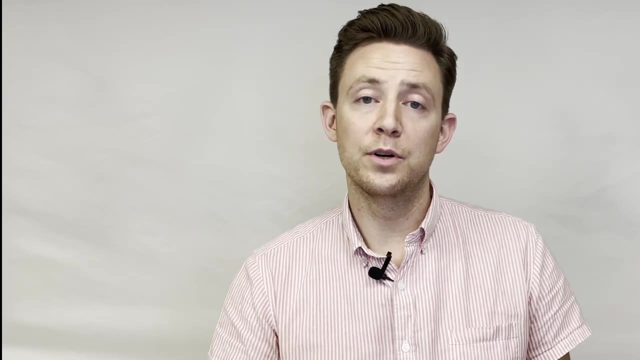 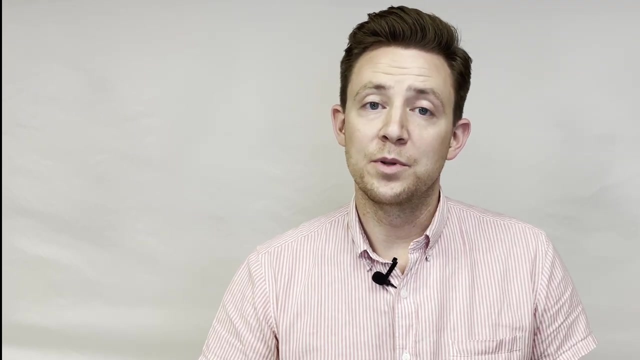 expert territory, but it's approachable enough to get started and for you to use, especially using more statistical models, for your GIS work. You could call the next course a book, an ebook, an online course- whatever you call it. It's awesome. This is the Geographic Data Science with Python book. This is also from Danny. 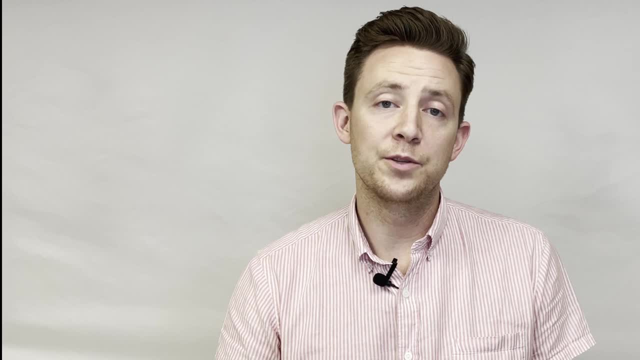 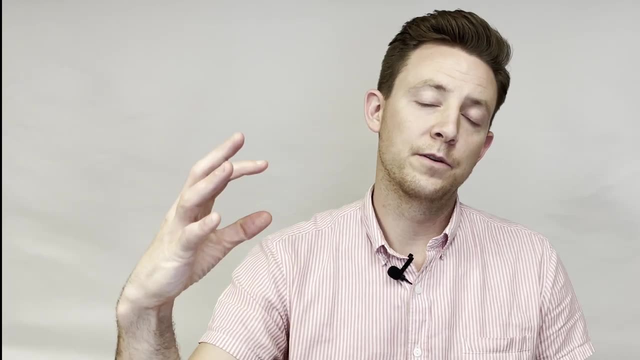 Arribas-Bell in our previous course and some other people that he's worked with on the Python Spatial Analysis Library: Sergio Rey and Levi Wolf. This is your next level up if you're looking to get into spatial data science. Dives into some more advanced concepts, really dives into the underlying. 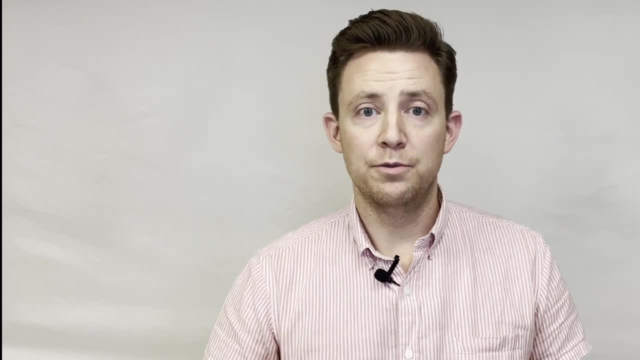 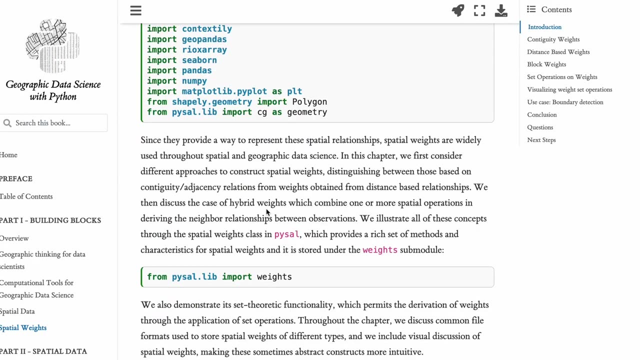 statistical models that are used in these tools, but also is very explainable, readable and, ultimately, approachable. I would recommend some understanding of statistical models, but it's not totally necessary, as they do an amazing job explaining what's actually happening in the tutorials. As you can see here there's more. 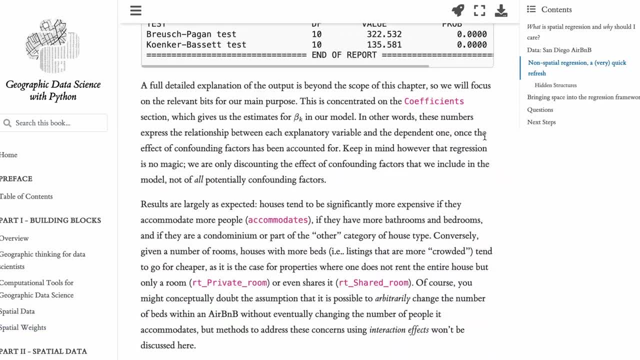 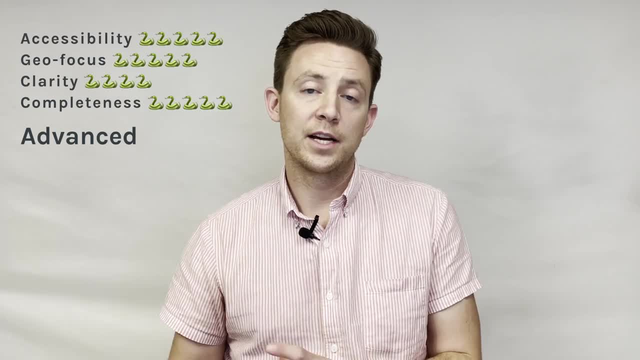 advanced topics like spatial regionalization or creating territories, spatial feature engineering, regression and deeper dives into other topics. I definitely rank this in more of the advanced or expert category, but it is an excellent resource and, as you start to ramp up, this is one you need. 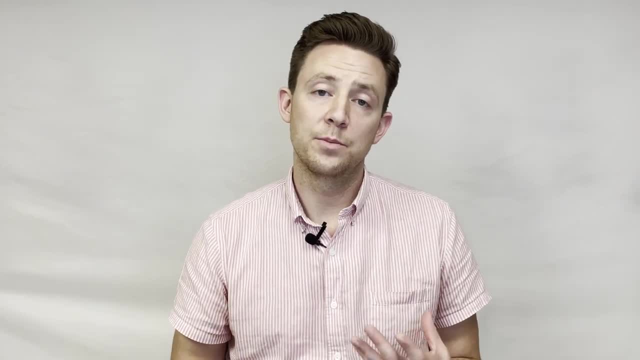 to check out. The next course is called an Introduction to Python Scripting for Geospatial. It was taught by Danny Arribas-Bell and Levi Wolf and he's going to give you a little bit of a tour of the course. 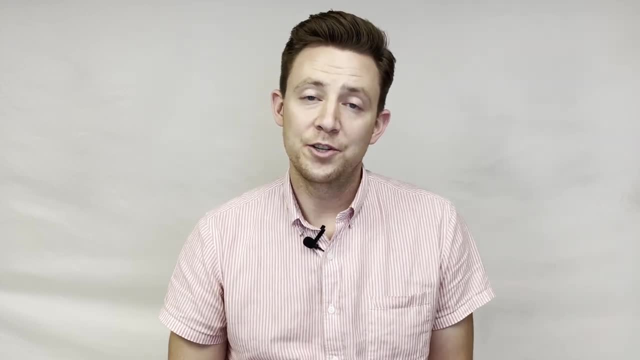 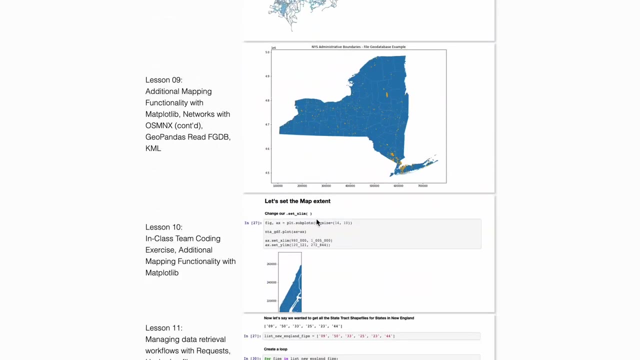 I'm Daniel Sheehan at the Pratt Spatial Analysis and Visualization Institute, or Pratt Savvy, in New York City in 2020.. I think this is an excellent resource. It was built for online learning and I think it's one of the most complete end-to-end courses I've seen on all 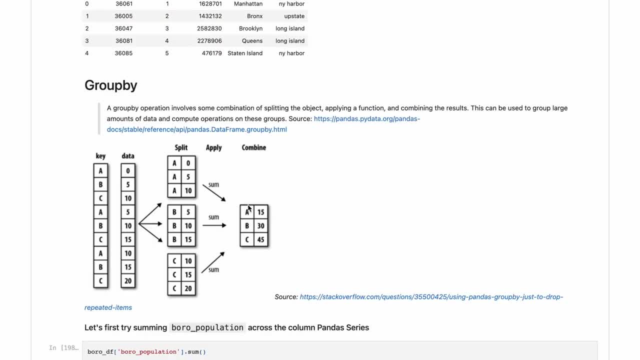 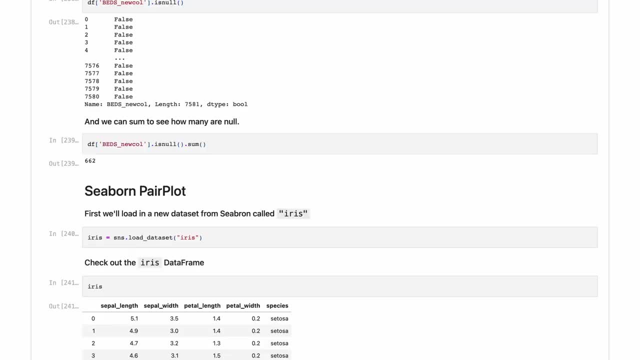 topics around geospatial Python, So it's meant to go along with the class and lecture, but if you follow along, you can understand most of the tutorials and work your way through it. That said, it's backed up with complete notebooks and tutorials on lots of different topics. This covers everything from 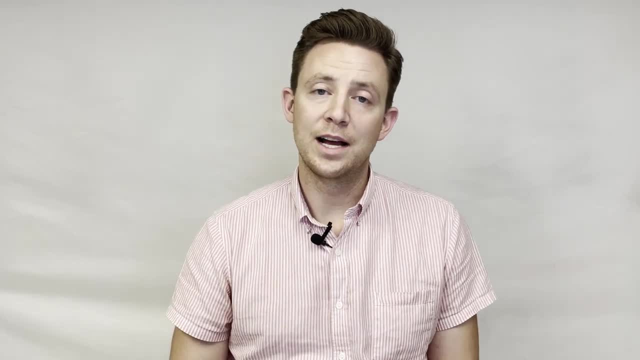 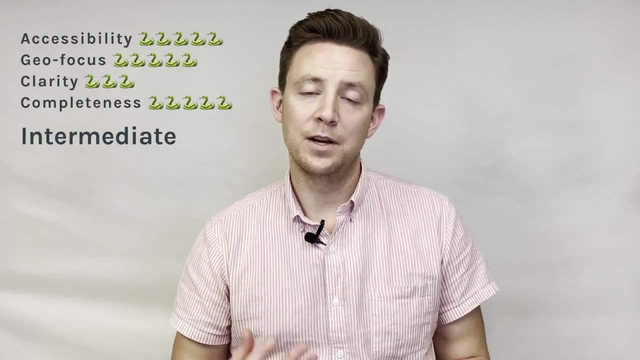 basic tools all the way up to more advanced things like network analysis using geocoding and lots of lots more, Definitely rank this in the intermediate category, but it's an amazing course for you to advance and go into different topic areas too. The next two courses come from one of 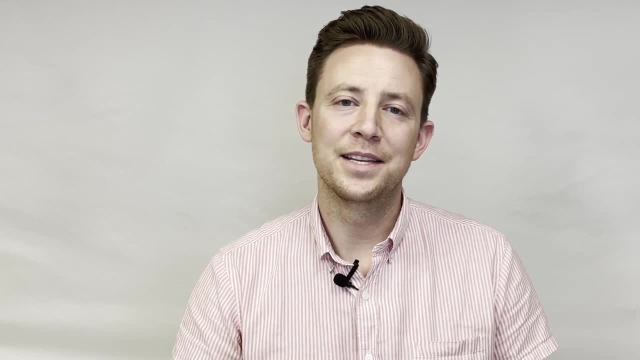 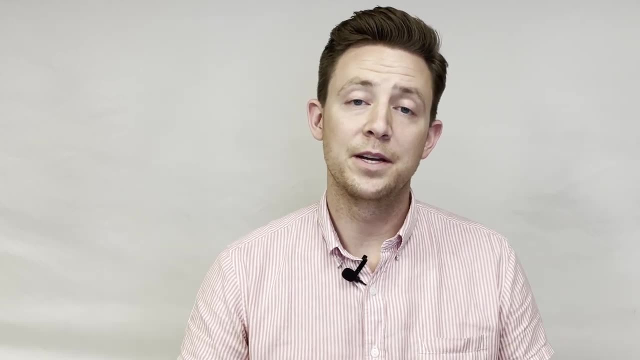 the best writers on all things geospatial Python and spatial data science: Abdi Shakur Hassan, who writes amazing articles on Medium and across the web. These two courses both live on Udemy and cover different topics around spatial data science and geospatial Python. If you're more of a 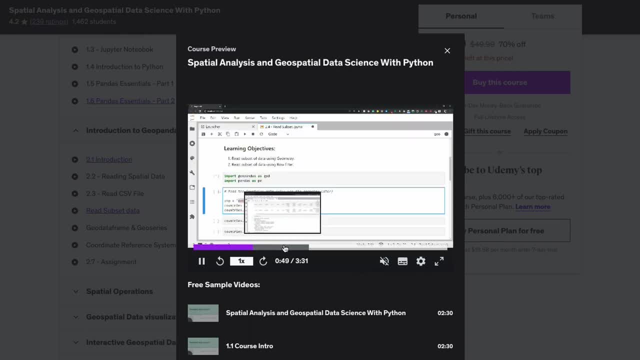 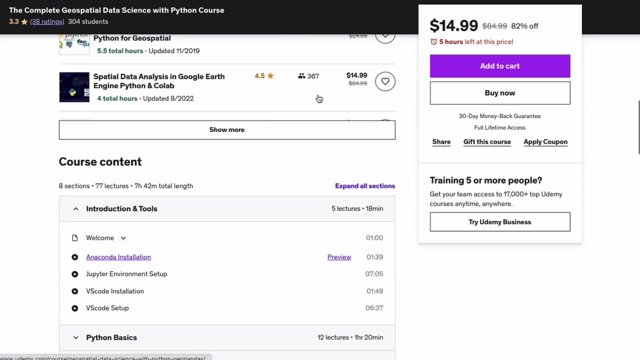 visual learner and like following along with videos and tutorials. I definitely recommend checking these out. These are paid courses, so do keep that in mind, but I think they give you a very poignant and fast track to learn some of these different topics. These courses also dive into 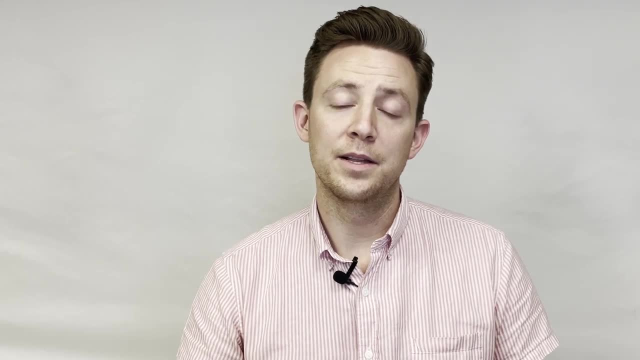 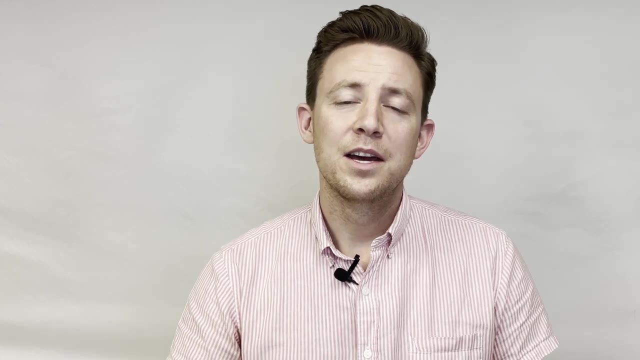 some different areas, like creating web apps from Streamlit, which you can do in Python, and other tools like Shapely and Fiona for manipulating geometries. Some of the other courses haven't dived into these quite yet, but I think there are really practical applications for. 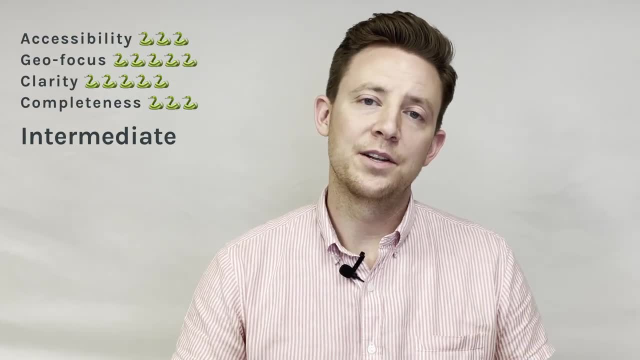 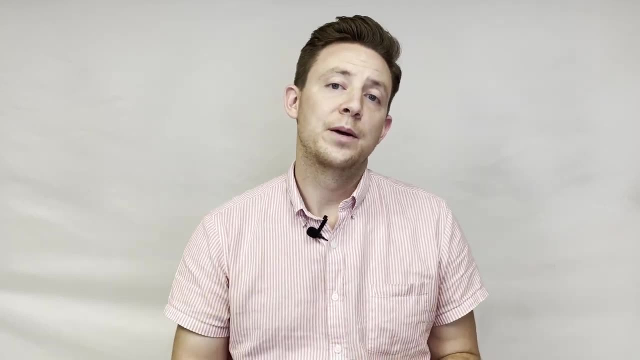 these tools too. These range from beginner to intermediate, so check this out and see if any of these might be right for you. As an aside, if you are looking for some different tools that focus on generic data science, this course from Udemy is actually one I use to learn. 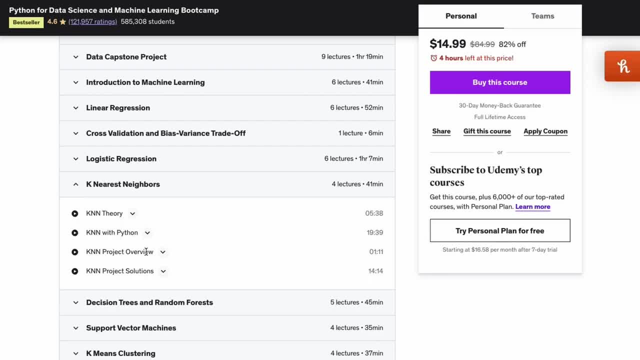 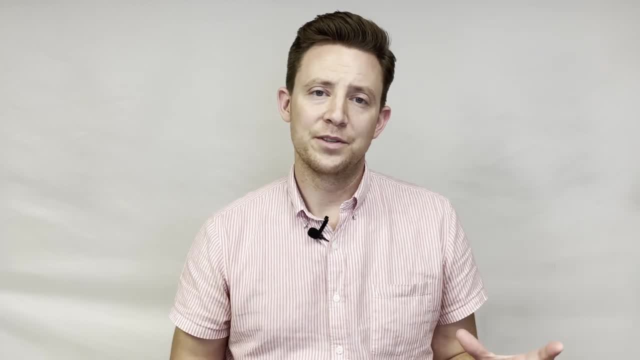 a lot of data science fundamentals. It gives you a lot of base learning in Python, but also dives into machine learning using different tools like scikit-learn and really helps you understand how to do these models as well. Now you can use a lot of geospatial data within machine learning. 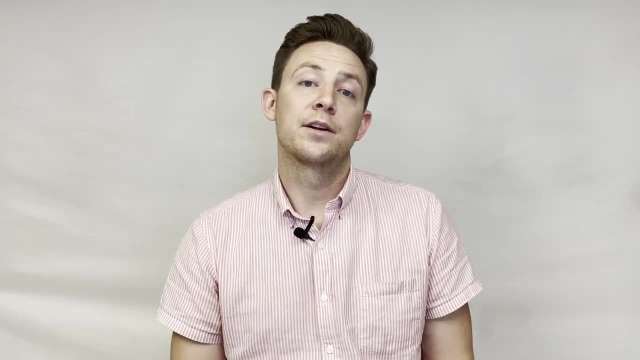 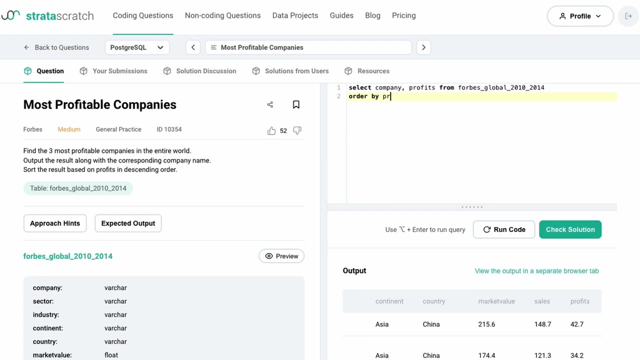 and I think this is a great place to start. I also recommend checking out Stratascratch. This is a great tool that gives you practice questions for topics in data science and SQL, and I think it helps you get some practical base if you are